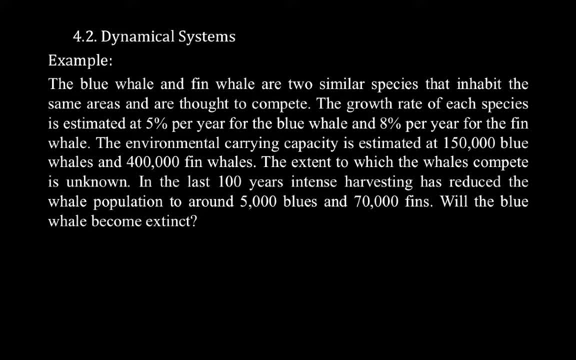 In the last 100 years, intense harvesting has reduced the whale population to around 5,000 blues and 70,000 fins. Will the blue whale become extinct? We are going to follow the five-step method, As we know the first step. we should define our 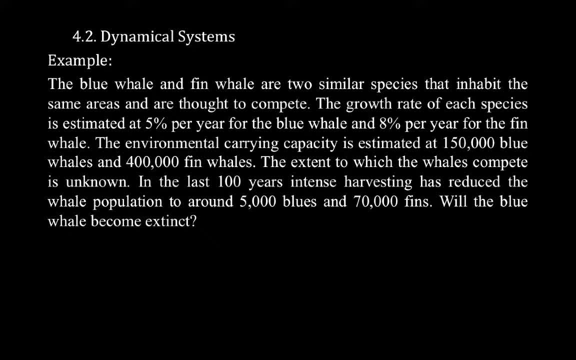 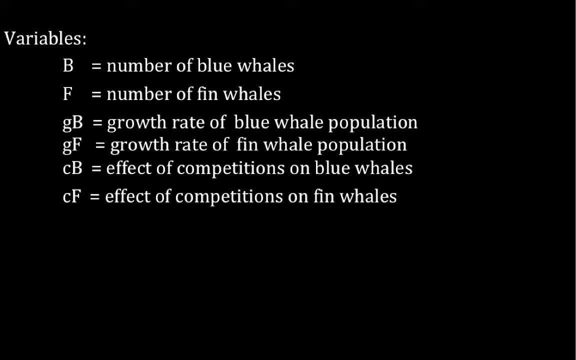 variables and assumptions. then objective: Choose B number of blue whales and F number of fin whales. GB and GF growth rate of blue whales and fin whale population respectively. CB and CF. effect of competition on blue whales and fin whales, respectively. 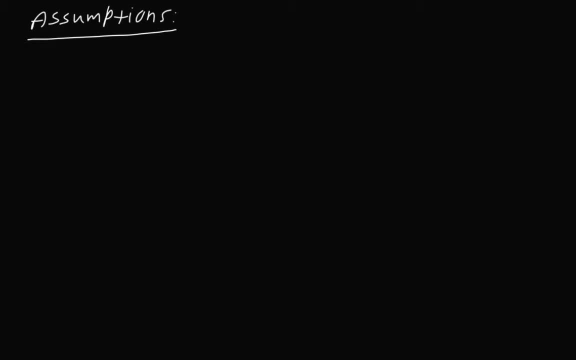 Now assumptions. Before I explain the assumptions of the example, Let me give an example Assumptions equation. we use this equation for the growth rate of population, P equal RP time, 1 minus P over K. so R is the rate, the rate at which the population would. 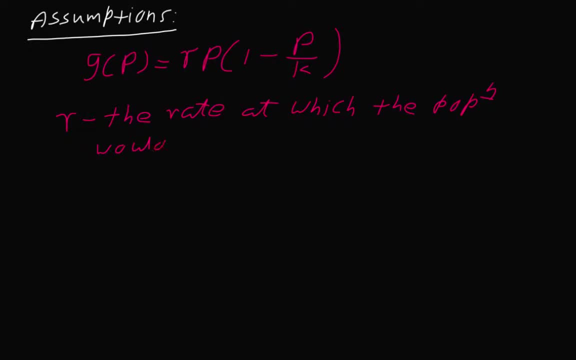 keep would keep growing in an unlimited environment. environment right, and K. K is the maximum number of individuals that the given environment can support, the maximum number of individuals that the maximum number of of individuals, individuals that the given environment can support. okay, we need this equation for this. 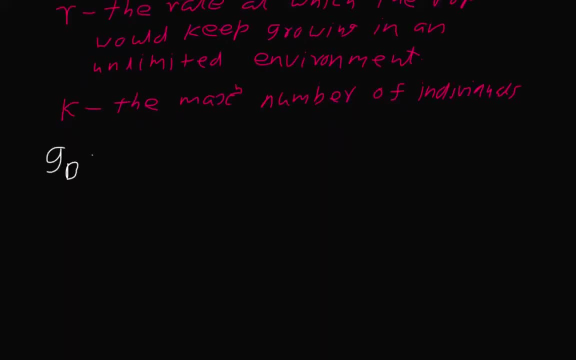 example, we use GB for the growth rate of blue whales population. so let me write down an equation for that this. so, according to the above equation, our are equal five percent. you see in the example, the intrinsic growth rate of each species is estimated at five percent per year. so therefore, are equal. 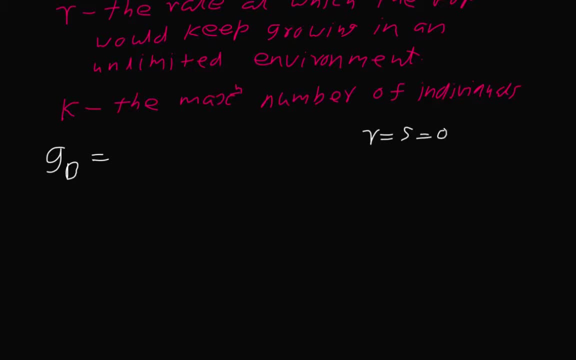 five percent, which is five percent you, which is 0.05, and K for this case. it's explained the example: the environmental carrying capacity is estimated at 150,000 blues. okay, 150,000 is the K, so now you can plug this numbers, so 0.05, so b we use here, B the blue. 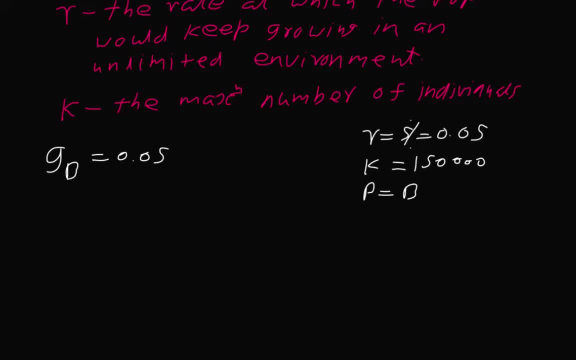 последs population. therefore I will use B over here, then one minus B divided by 150000. so same thing we can write down for the GF and B for thing it. this is the balance of graphic ward. so so what we hear is low. we also heard one underscore plus 0.05. so the Cargos that we will find out when. пять percent of the values was number, our gains are hundred kinds water versus that on the increase and we also will see an axis, so a strong balance of velocity of the values and then devam as normal balance. this only divided by 30, plus of order in our information furniture as to draw. it will start as to that in. 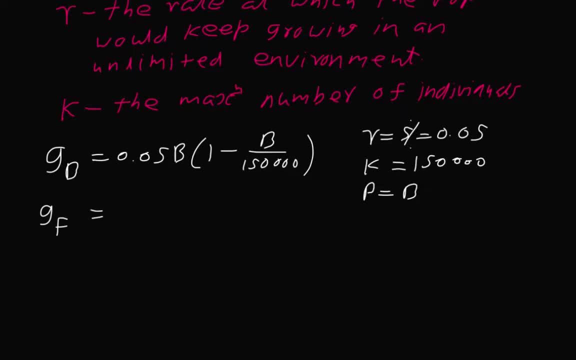 yes, there are some other post card here if you like. I think here we will see the for the fin whales, this one: 8%. Please read the example again. It's say 8%, which is 0.08, then F 1 minus F, what is the maximum? 400,000.. Therefore 400,000.. So these are the two assumptions. 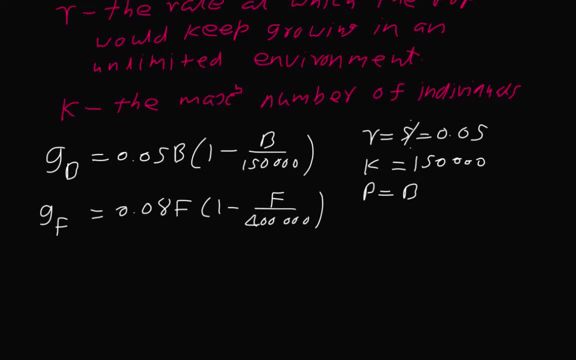 and also Cb effect of competition on blue whales and the fin whales. both must be equal. So we can write down. I use the alpha, it's just a positive real constant. So we can write down alpha times, Bf. So you know very clearly Bf. 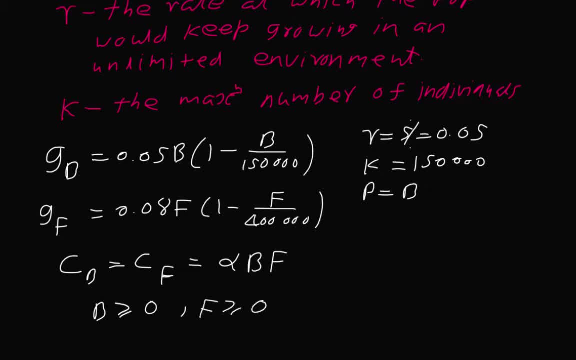 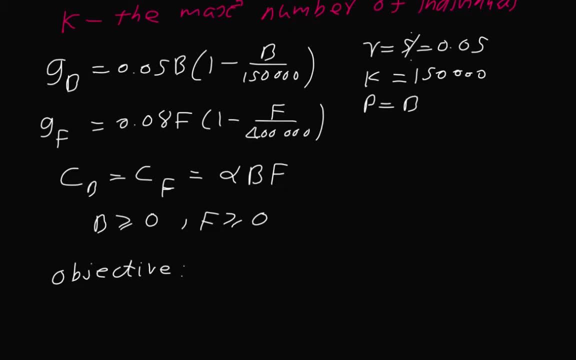 greater than or equal to 0 and F greater than or equal to 0.. Then objective: determine whether dynamic system can reach stable equilibrium starting from B equals 5,000,, F equals 70,000.. Now is step two. step two is to select the modelling approach. We will model this problem. 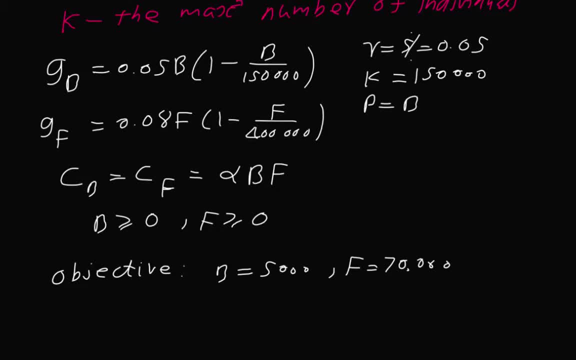 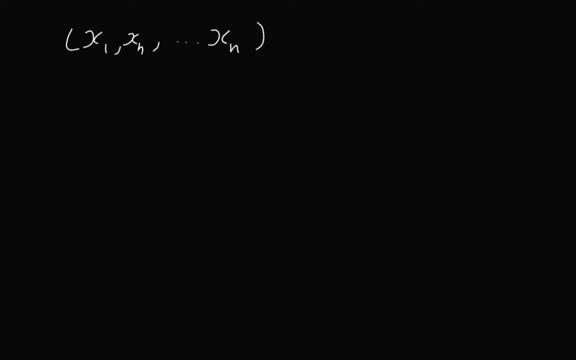 system. so, like last time, we can see the n state variables. then we do have functions f1 to fn represent the rate of change. so I will write down same function: f1, X1, X, N. this f1 is the rate of change of variable X1. 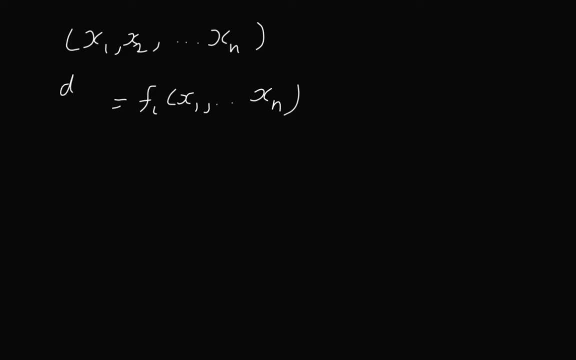 therefore, you can write down the D or Dec rate of change of the variable X1. similarly, you can write down, up to ndxn or ftfn: x1, Xn and differential equation, actually a system of differential equation. so you know, X 1, X, n is in s, s is a subset of RN. you can write down the point X, X, 1, X, n. 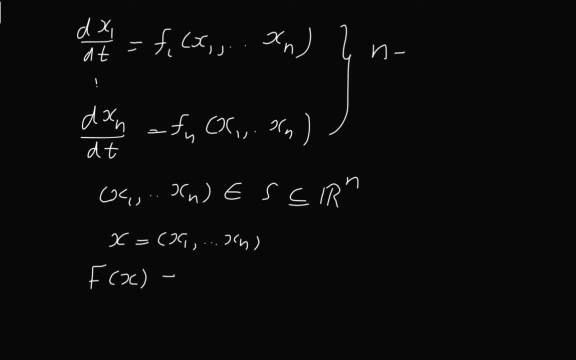 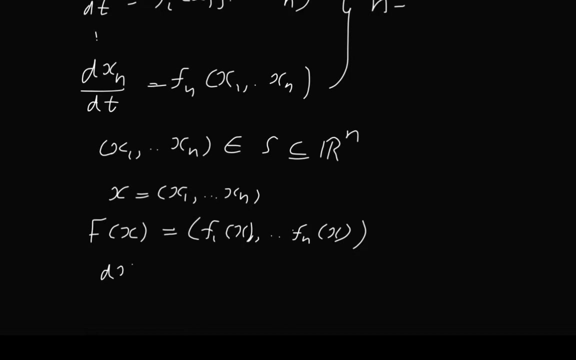 fx equal f1 a fnx, then the dynamical system equation can be written: the X over DT equal fx, which is f1 X fnx. the points where fx equals 0 are the equilibria and we will pay special attention to the vector field nearby this point. I will explain this in a step. 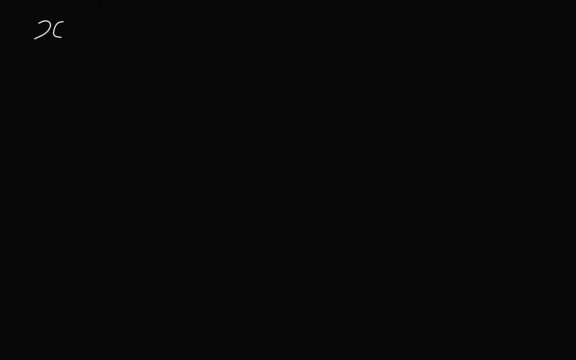 3. so step 3 is to formulate the model as last time. we use X 1 equal B and X 2 equal F. then we can write down the functions: X 1, prime equal f1. X 1, X 2- f1 represent the. 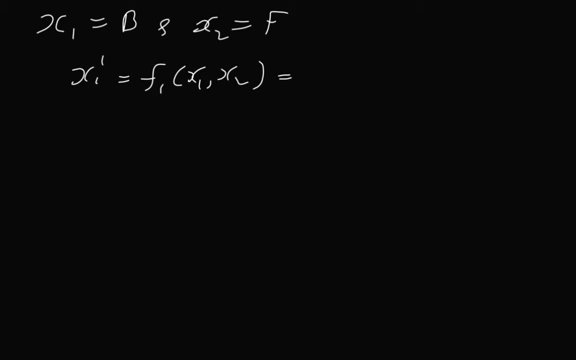 rate of change of X 1, according to our assumptions, you can write down f1 GB GB minus CB. once we plug the X 1 and X 2 GB can be written 0.05 X 1- 1 minus X 1 divided by 150,000, you can write the CB. 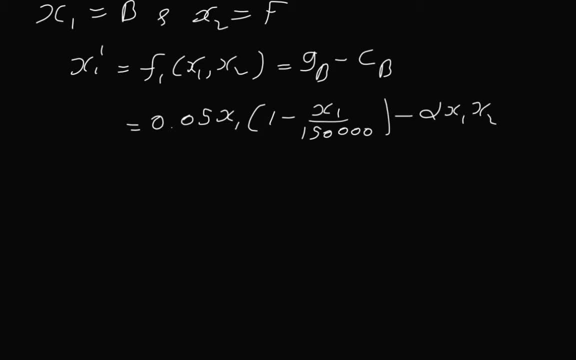 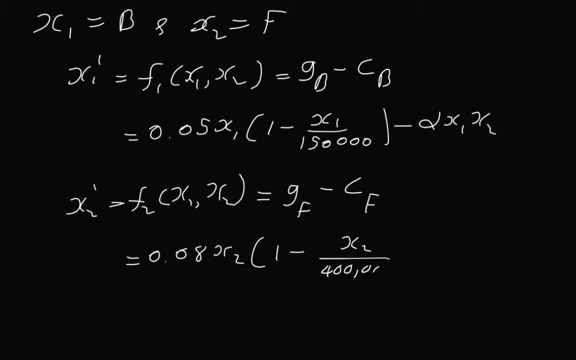 alpha X 1 X 2, X 2. prime, which is f2 X 1 X 2, can be written GF minus CF, so equation should be 0.08 X 2, 1 minus X 2 divided by 400,000 minus. 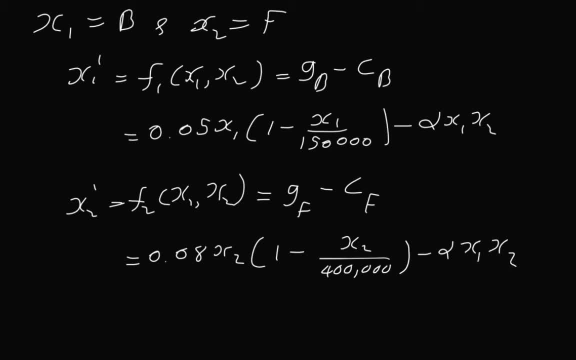 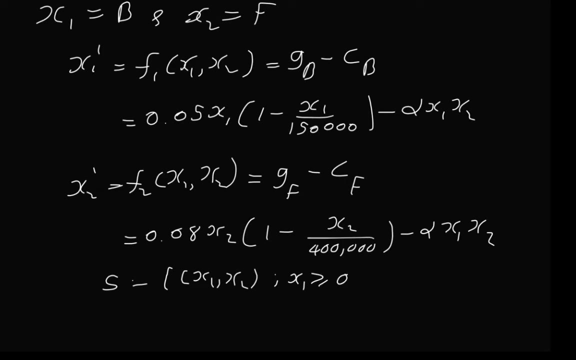 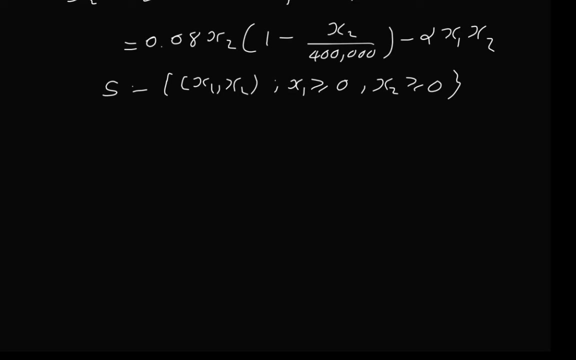 alpha: X 1, X 2. so you know the state space which is s and equal X 1, X 2, because we do have only two variables: X 1 greater than or equal 0, X 2 greater than or equal 0. so next is step 4, which is to solve the model. so 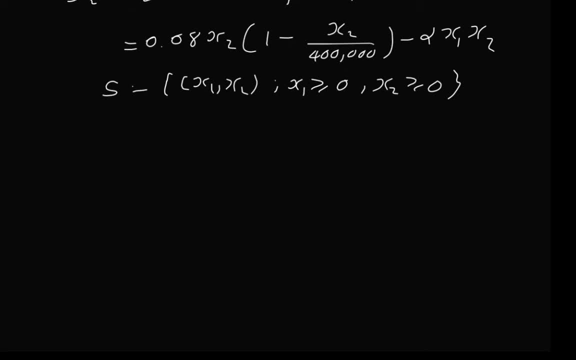 how do we solve model? as I mentioned before, we use the graphical method. let me draw the graph of pinwell. and so X 2 versus blue whales, so X 2 versus X 1. if you consider the graph, f1 equals 0 and f2 equals 0, you can get two graph like this. so you see, we should consider.